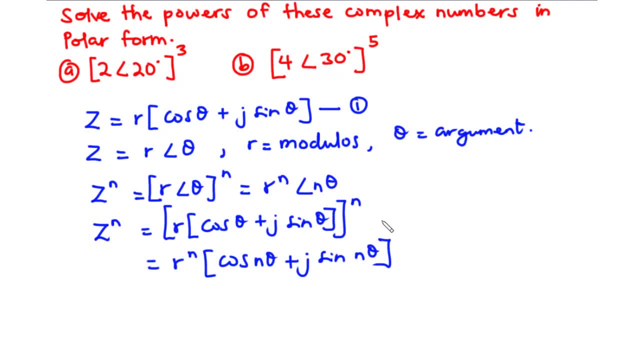 Solve the powers of these complex numbers in polar form. We have a: 2 polar 20, all cubed, and then 4 polar 30, all exponent 5.. Now let's solve these together. So for a, we have 2 polar 20, all exponent 3.. 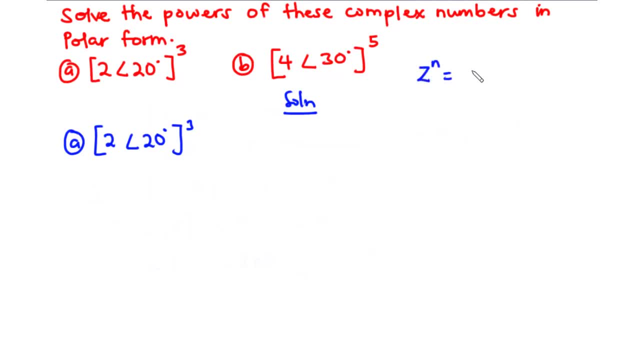 Now we said that given that z exponent n is equal to r polar theta, all exponent n, Then we simplify this as r exponent n polar n times theta. So let's apply this here. So this becomes r 2 exponent 3 polar 3 times 20.. 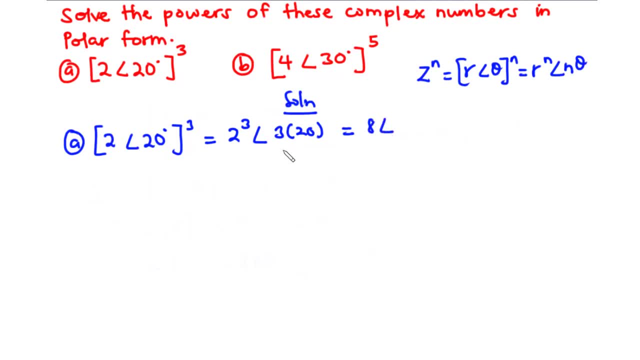 2 exponent 3 is 8.. So we have our answer to be 8 polar 60.. Now for b, we have 4 polar 30 degrees, all exponent 5.. So this becomes 4 exponent 5 polar 3 times 20.. 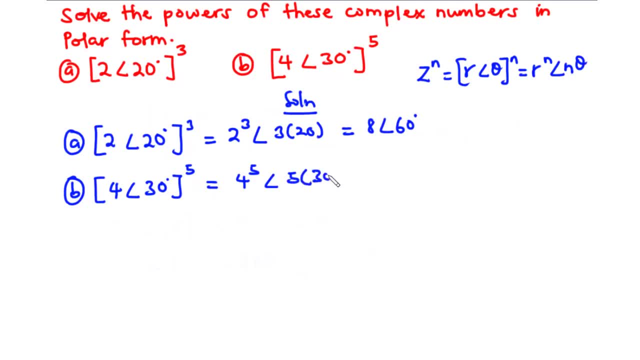 So this becomes 4 exponent 5 polar 3 times 20.. So this becomes 4 exponent 5 polar 3 times 20.. 5 times 30.. 4 exponent 5 gives 1024.. Puller 5 times 30,, we have 150. 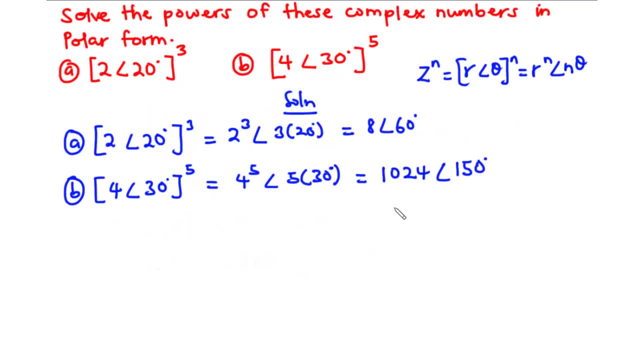 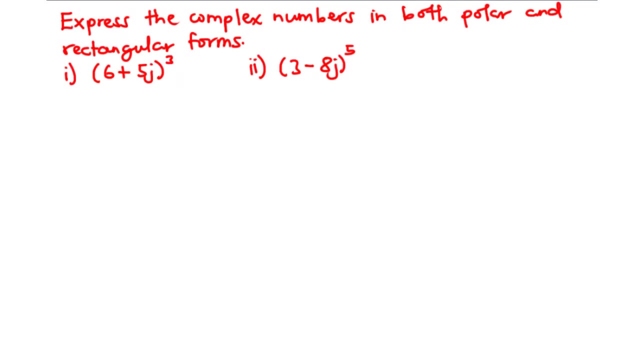 So that is 150 degrees. So basically, this is how to solve the powers of complex numbers. Now, in the next section, we are going to consider more complex examples. So let's try these examples together. Express the complex numbers in both puller and rectangular forms. 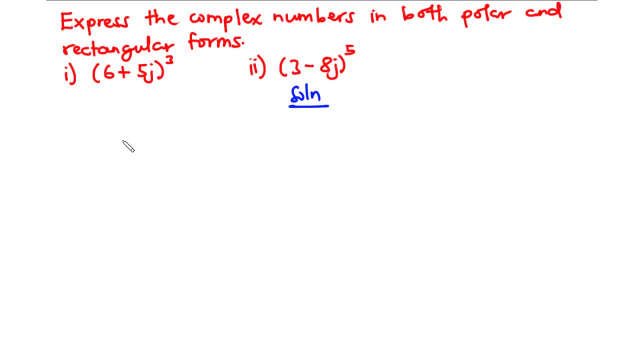 So here we have two complex numbers which are all in the rectangular form. So first of all we need to resolve these complex numbers in the puller form. Then we can use the Morbius theorem to solve the powers. 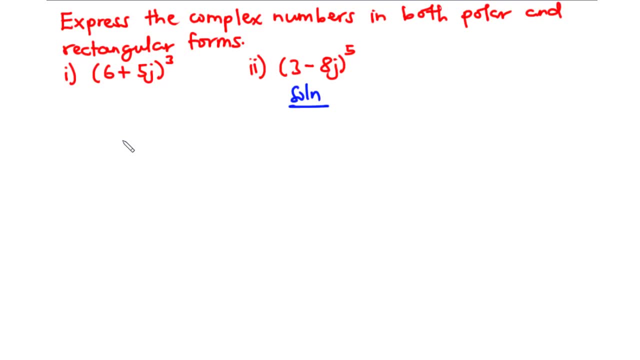 And then leave our answers in both puller and rectangular. So these are exactly what we are going to do. So let's solve for i. So for i we can say that let z equals 6 plus 5g. 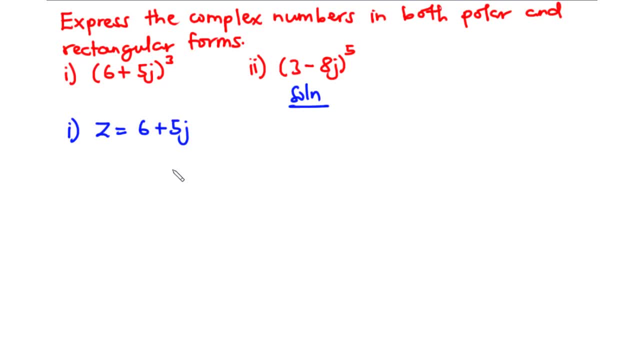 Now this complex number is in the rectangular form. We need to convert to the puller form. So we are going to draw the Argand diagram. We have the imaginary axis, We have the real axis. This is the origin. We have the x component to be 6.. 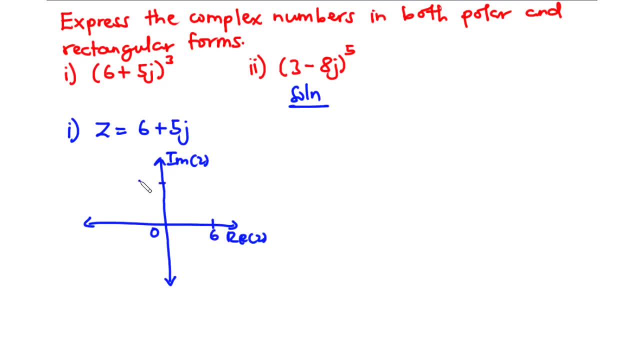 And the y component to be 5.. So it means that we have our complex number appearing in the first quadrant. So that is, z equals 6 plus 5g, This is r, And then we have the angle theta. 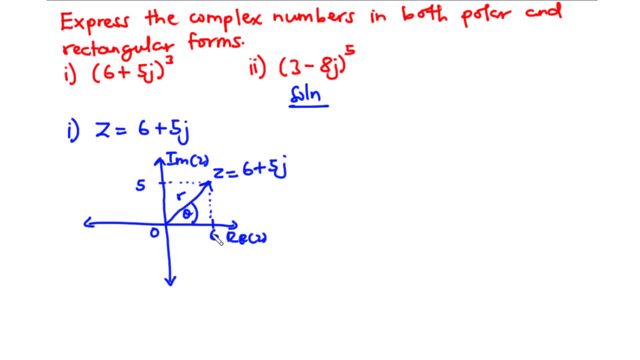 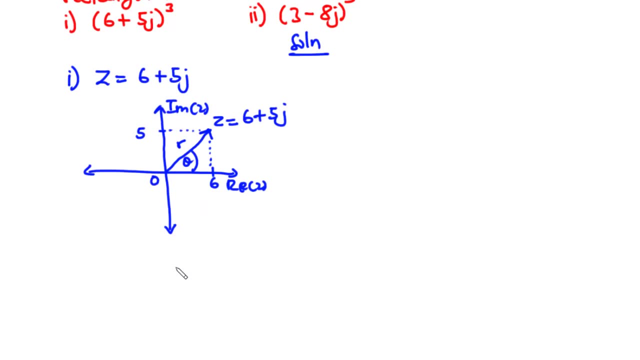 The angle theta formed between r and the positive x axis. Now let's find r, which is the modulus, And then theta, the argument. So we have: r equals the square root of x squared, plus y squared, We have x to be 6.. 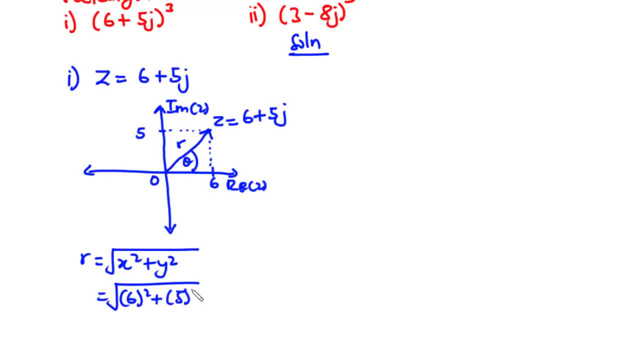 So 6 squared y to be 5.. 5 squared, 6 squared is 36.. Plus 5 squared is 25.. So 36.. So 36 squared is 25.. And that is equal to the square root of 61.. 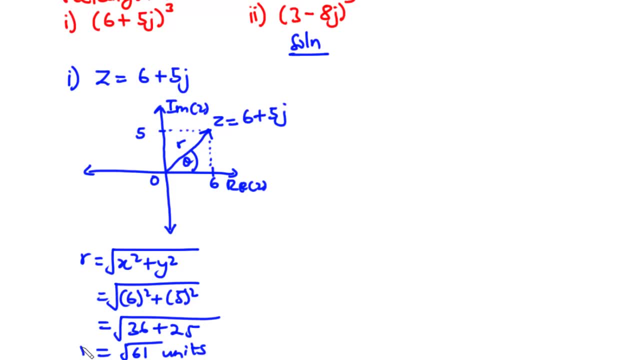 So we have the square root of 61 units, That is, the value of r. Now let's find the value of theta. So we have theta to be equal to tan inverse of the absolute value of y divided by x. So this becomes tan inverse of. 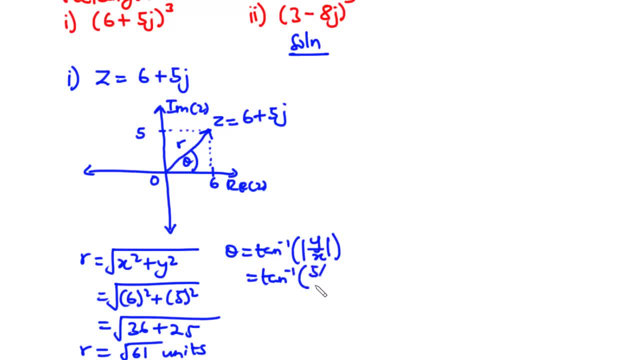 We have y to be 5.. And then x to be 6.. So tan inverse of, So tan inverse of 5 over 6 gives 39.81 degrees. So this is the value of theta. Therefore, our complex number z, equals 6 plus 5j, can be represented in polar form as square root of 61 polar 39.81 degrees. 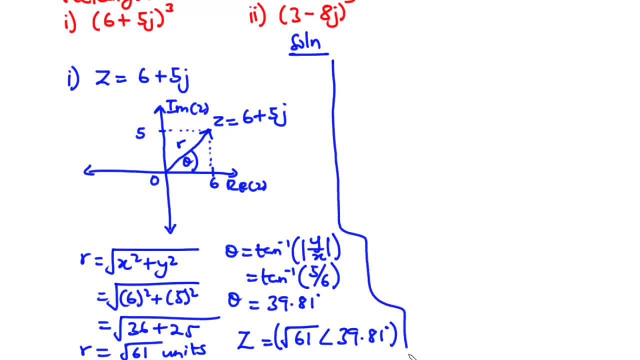 So, according to the Morphe's theorem, z exponent n is equal to r exponent n polar n times theta. So in our case, z exponent 3 is equal to the square root of 61 exponent 3 polar 3 times 39.81.. 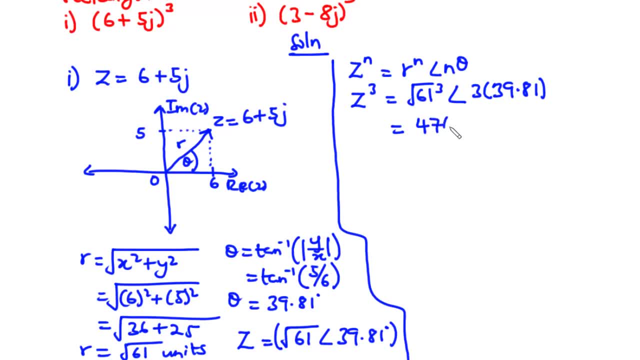 And that gives 476.43 polar 119.43.. So basically we've been able to represent this complex number, that is 6 plus 5j, exponent 3, in the polar form. So this is the polar representation of z cube. 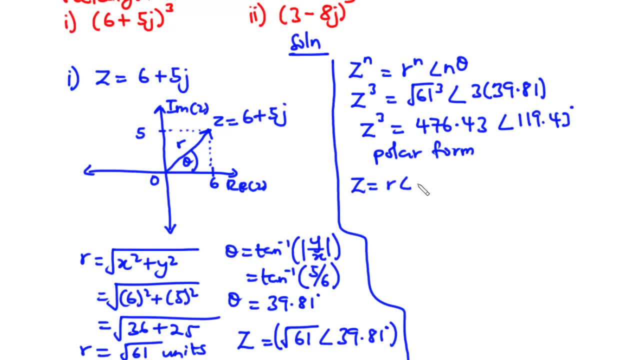 Now, since z equals r, r polar theta is equal to r cos theta plus jr sine theta, Then we say that z cube is equal to, We have r to be 476.43.. So 476.43 cos the angle that is 119.43 plus j times 476.43.. 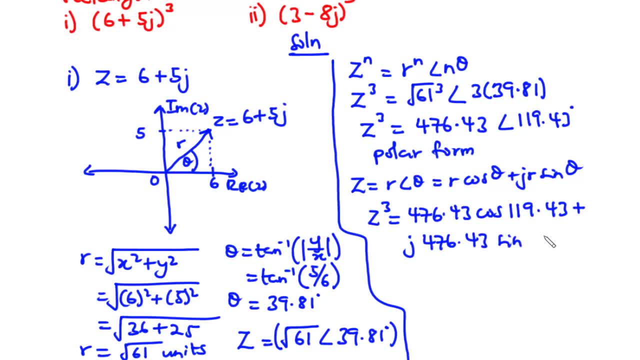 Sine 119.43.. So finally we have z cube equals 476.43. cos 119.43 gives negative 234.10.. gives j times 414.95.. So this is the rectangular representation of the complex number. Now. 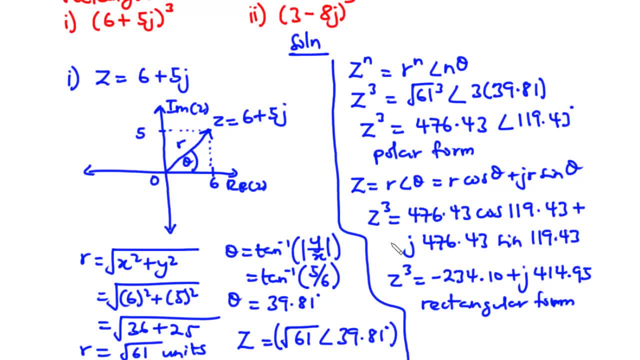 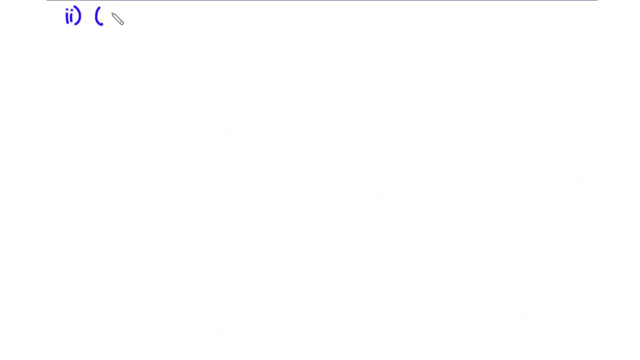 let's move on as we solve for ii. So for ii we have the complex number 3 minus 8j, all exponent 5.. So let z equals 3 minus 8j. Therefore we need to represent this in the polar form. 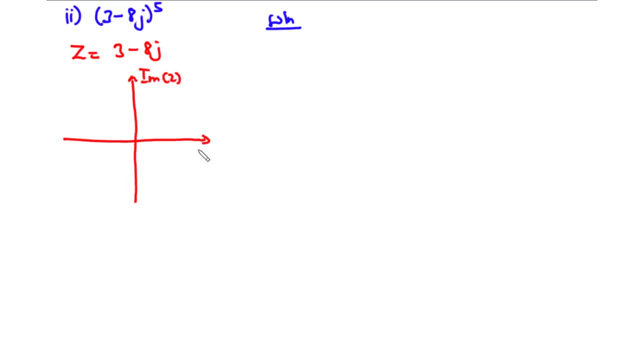 We have the x component to be 3.. So that is 3 and the y component to be negative 8.. So negative 8 is here, which means that we have our complex number z occurring in the fourth quadrant. So let this angle be alpha, that is, the angle formed between r and the positive x axis, taking 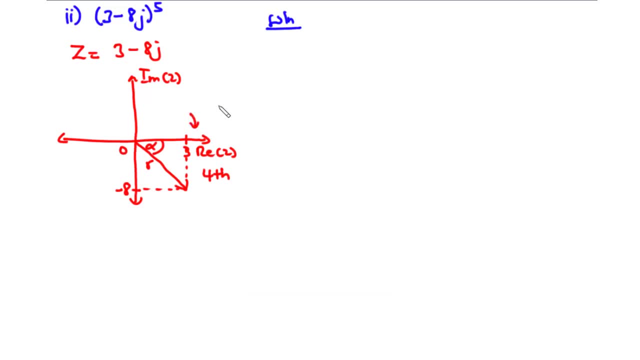 in the clockwise direction. So first of all let's find the value of r. So r is given by the square root of x square plus y square. we have r equals the x component is 3, so we have 3 square plus y component: negative 8, so we have negative 8 square. 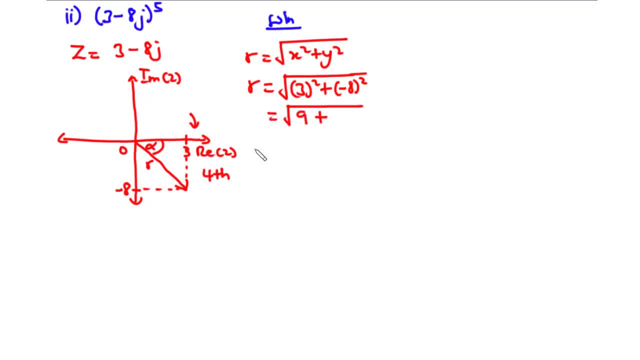 3 square is 9, plus negative 8 square is 64.. So 9 plus 64, we have 73,. so that is the square root of 73 units. Now let's find the angle alpha. So alpha is given by: 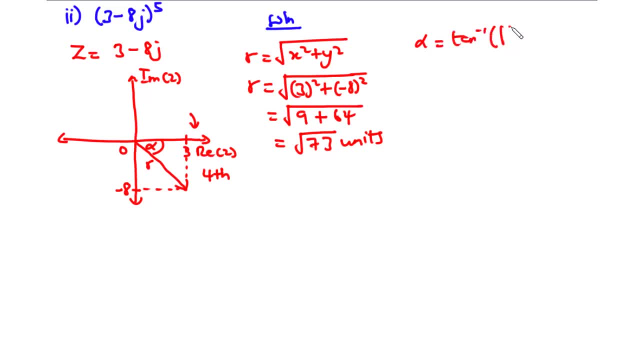 Tan inverse of the absolute value of y divided by x, We have tan inverse of y. that is, the absolute value of y is 8, and then that of x is 3.. So tan inverse of 8 over 3 gives 69.44 degrees. 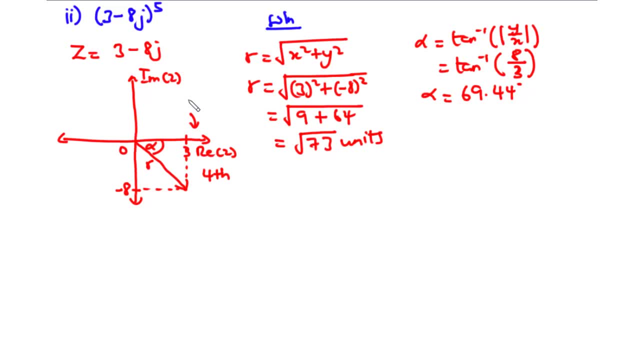 So this is the value of alpha. Now, since we are interested in finding the angle Formed between The positive x axis and r taking in the anticlockwise direction, that is, this angle, We are going to subtract alpha from 360.. 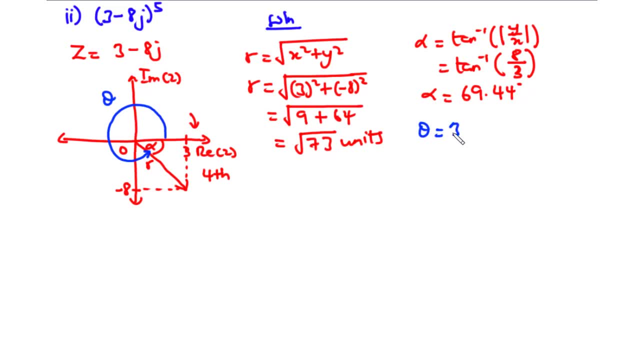 Therefore, we say that theta is equal to 360 degrees minus alpha, which is 69.44 degrees. Now the reason why we are going to subtract alpha from 360 is that we are interested in the angle formed between the postive x-axis and r taking in the anticlockwise direction. 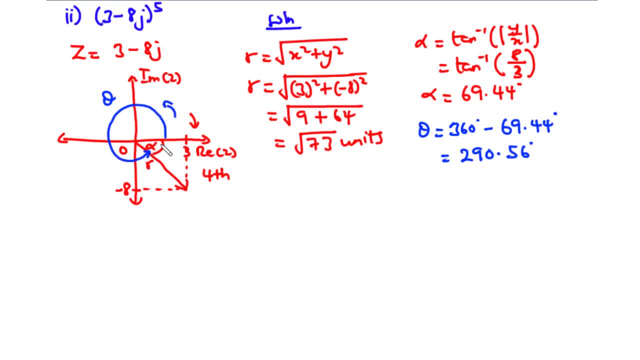 so from this point through to this point is 360 degrees. Now, since we are interested in the angle formed between this point 3 to this point, If we know the full angle, which is 360.. Then we want to subtract the small angle from 360 degrees minus alpha, which is 61 degree. 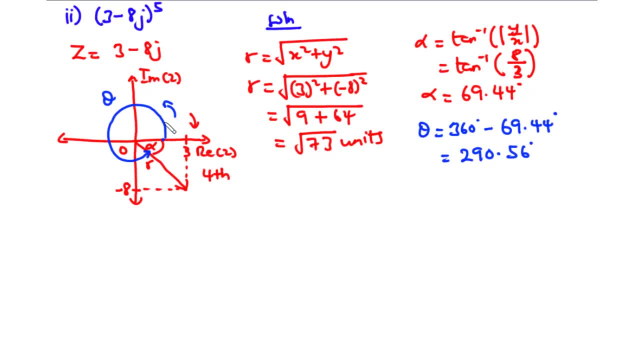 The angle, which is 5 degree. 360 degrees minus alpha, equals pongu. approximately details from 360 to get the angle theta. so we have theta equals 290.56 degrees. therefore z in the polar form is represented as the square root of 73 polar 290.56 degrees. so this is the 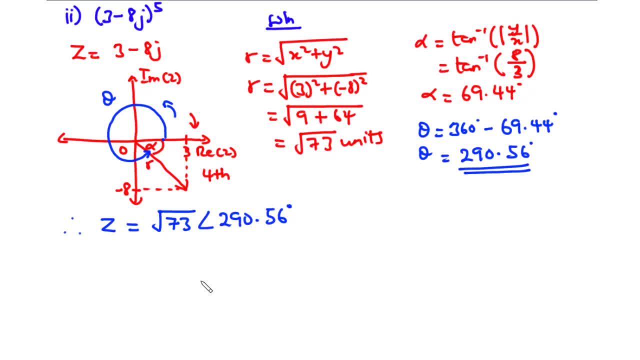 value of z. now we are interested in expressing z exponent 5 in the polar and rectangular forms. so in the polar form we have: z exponent 5 equals the square root of 73 exponent 5, polar 5 times 290.56 degrees. so the square root of 73 exponent 5 gives: 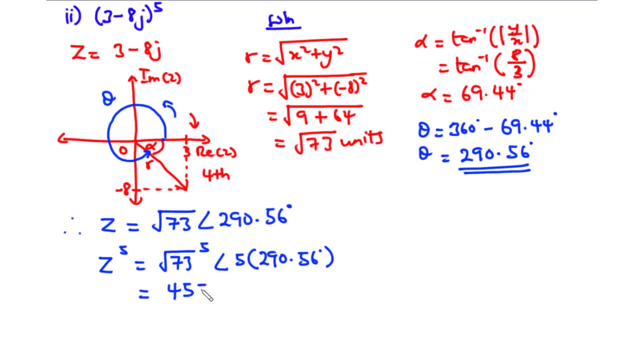 z 45 531 polar. 5 times 290.56 gives 1452.8 degrees. now the value of theta was found to be 1452.8 degrees. now this angle is greater than 360 degrees, so we need to subtract 360 degrees from this value. 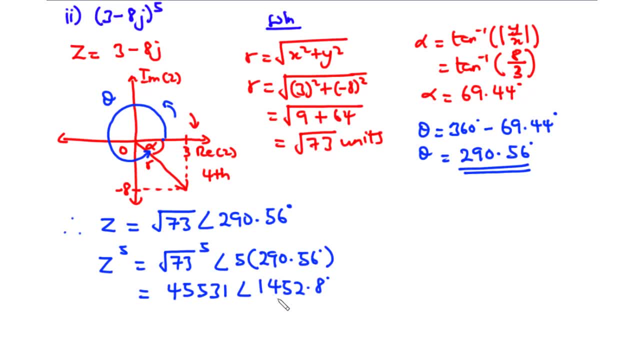 as many as we can until we get a value that is less than 360 degrees. therefore, 1452.8 degrees minus 4 times of 360 degrees gives 12.8 degrees. so we can simplify this as 12.8 degrees. so that is what we are going to use.